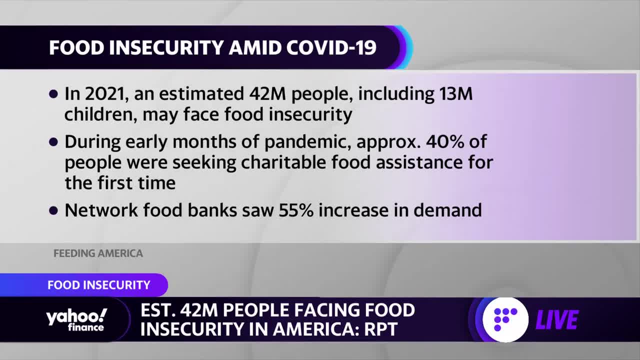 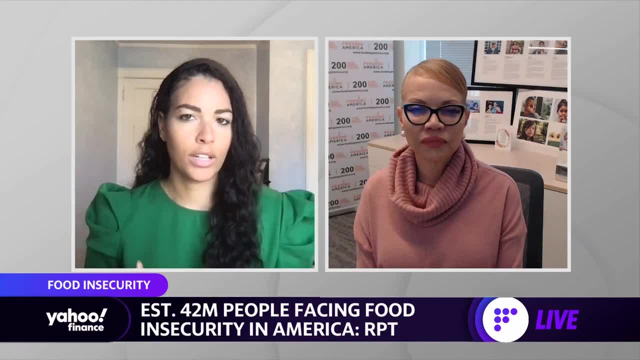 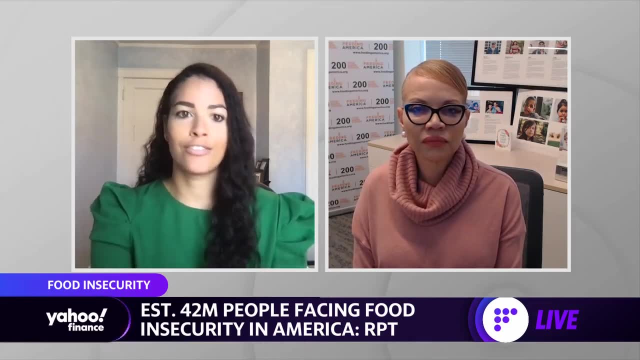 recovery if all holds. that's doable. I think it's going to require an all-in fight, but I think we can do that. I want to talk about innovation in this space. It's something that we talk often about throughout this pandemic from a lot of companies, how they have been forced to innovate. 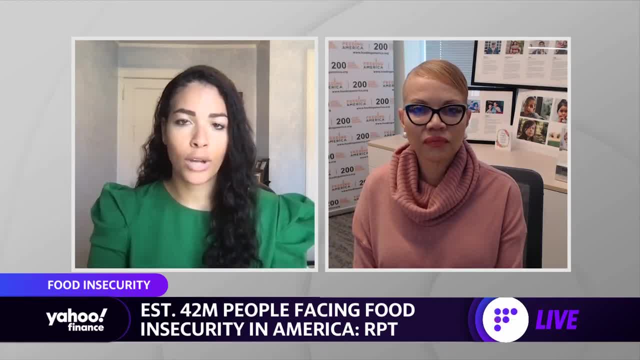 to stay competitive and stay afloat throughout the pandemic, And I was reading in the notes that food banks were similarly innovating throughout this pandemic to really help as many folks as possible get access to food. I'm wondering, looking out ahead, are there any lessons learned? 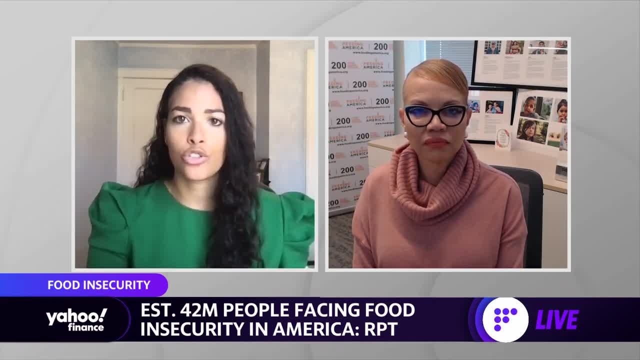 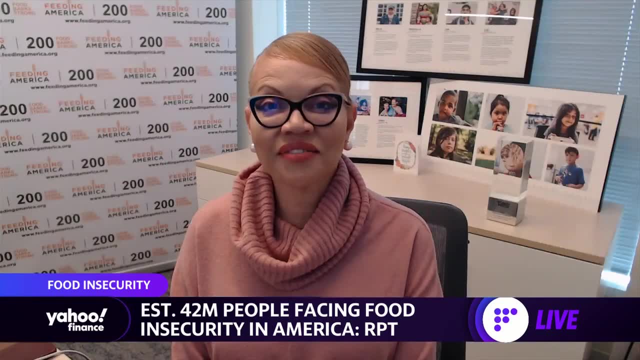 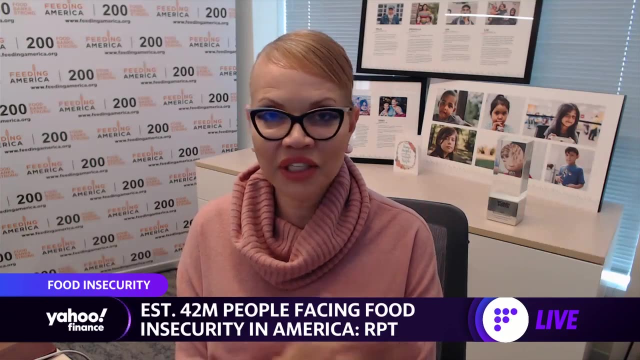 any innovations when it comes to food equity and distribution that can be used in this fight to essentially end hunger. Yes, there are. There are lots of innovations that we're going to be able to take, pull forward, or at least we're certainly going to try to. I should probably have said at the 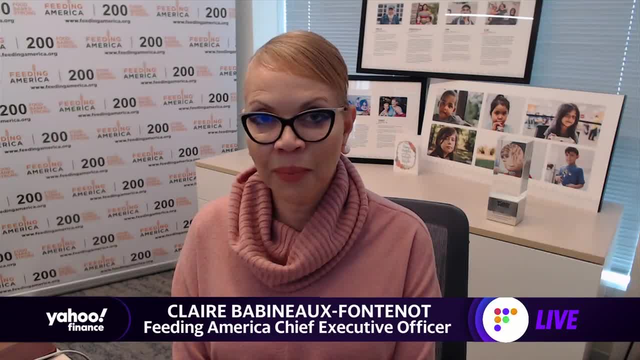 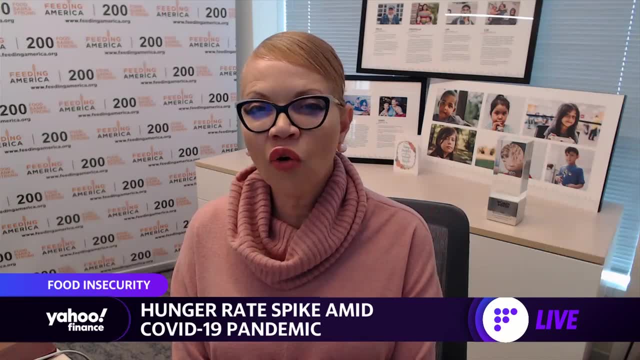 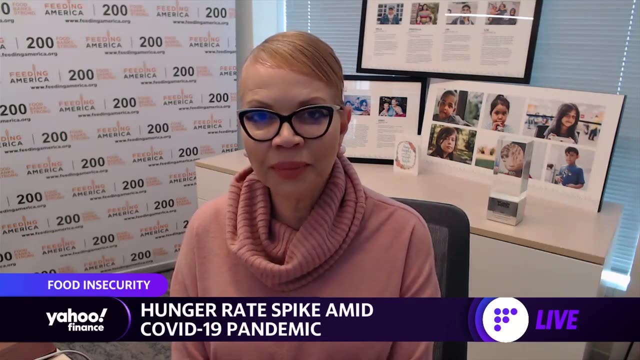 very top of the segment that we should be saying thank you to the American people. Because of the help, outpouring of support that we've had, we were able to provide over 6.1 billion meals last year. 6.1 billion meals: That's what lots of new partners coming to the table and lots of those. 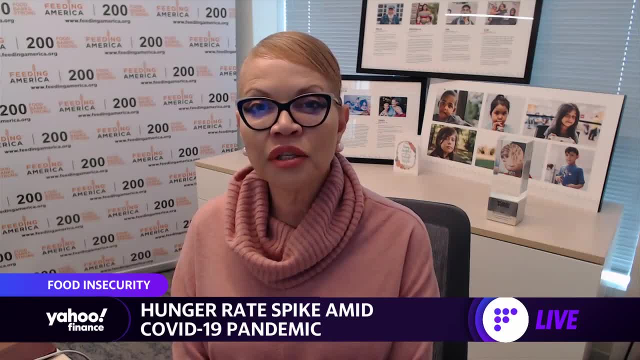 innovations have been a result of some of those new partnerships, So we're doing some new and innovative things about getting food equity and distribution. getting food equity and distribution directly to where people are who need it- A lot of people who face food insecurity especially. 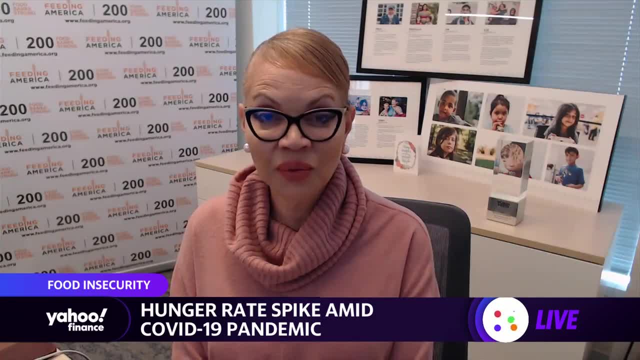 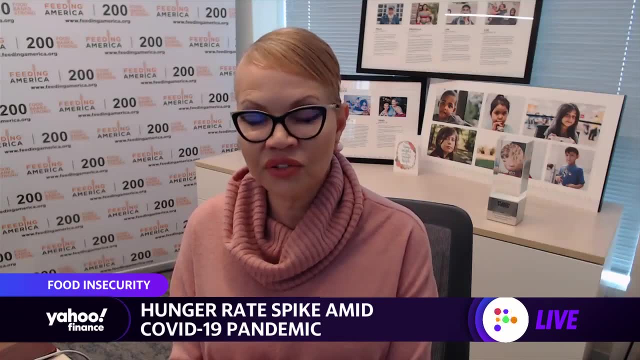 really deep food insecurity- don't have access to cars, So when you were seeing those long lines of cars out there, there are some people who can't even get to a car in order to get to the food. So we've had some creative things that we've done. We've increased the number of mobile 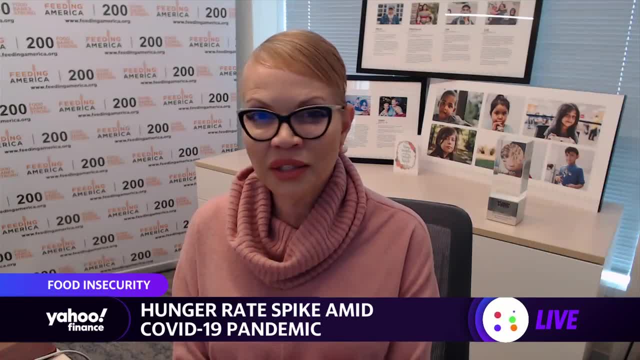 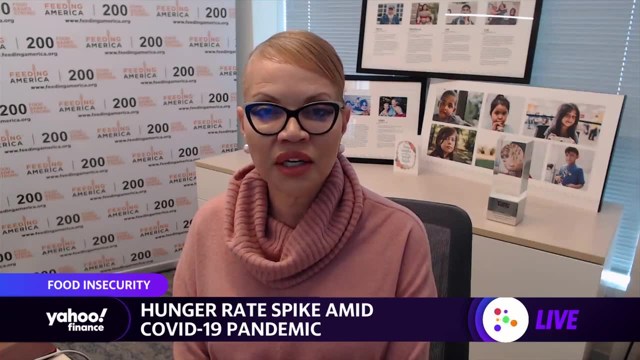 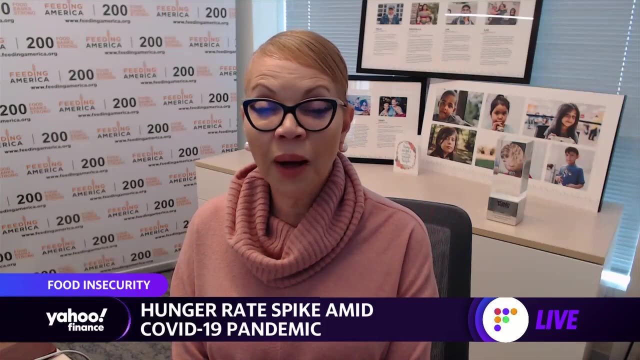 distributions, where we're going into rural communities. Lots of people in the audience may not be aware that there are some significant challenges around hunger in rural communities across the country, So we've been getting out farther and farther out to where people are who are in need of help. We've come up with, we've created new partnerships that we hope. 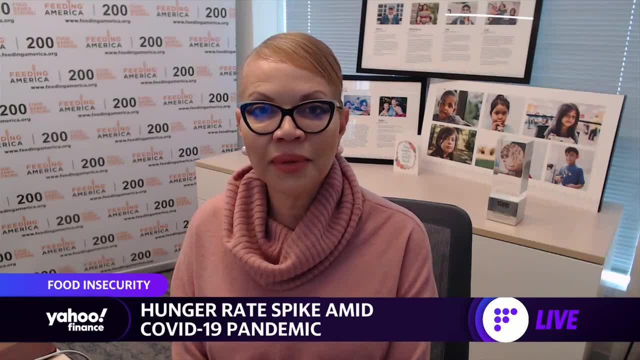 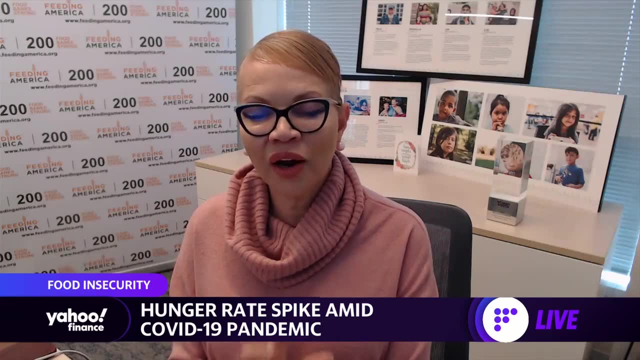 that we'll be able to bring with us beyond the pandemic. And I think if we continue to trigger those innovations, if the American public continues to open their hearts and minds to this real big challenge that people are confronting, I'm confident that we can make. 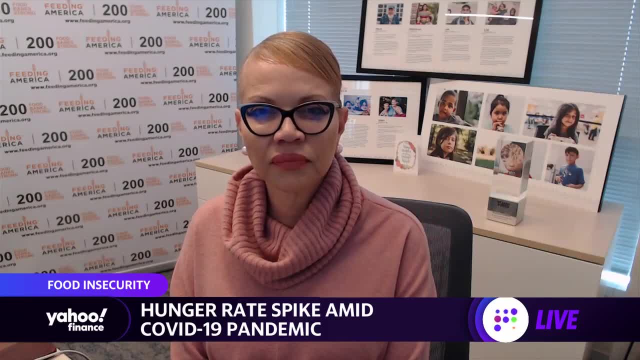 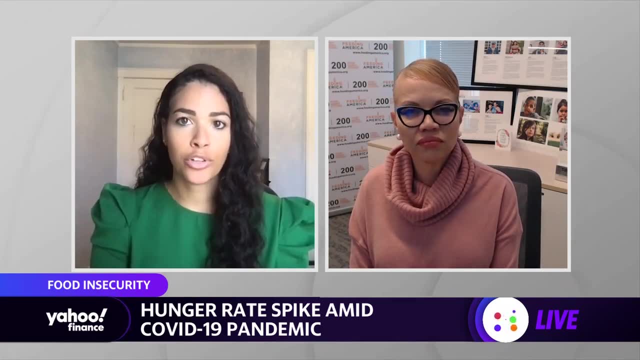 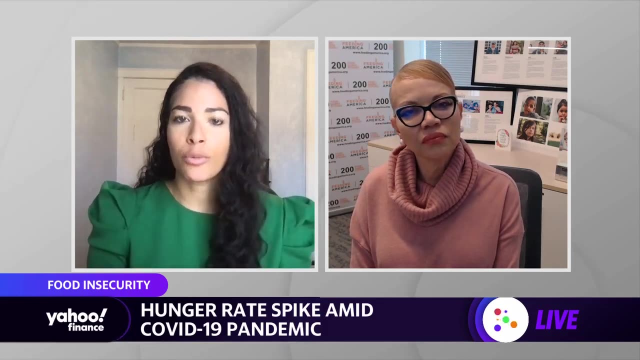 a whole lot of progress going forward. Now you were mentioning how so many Americans you know opened up their wallets and their pantries to really help their neighbors, their communities, even folks that they did not know, essentially get through this pandemic with some food. But of course, the federal government also. 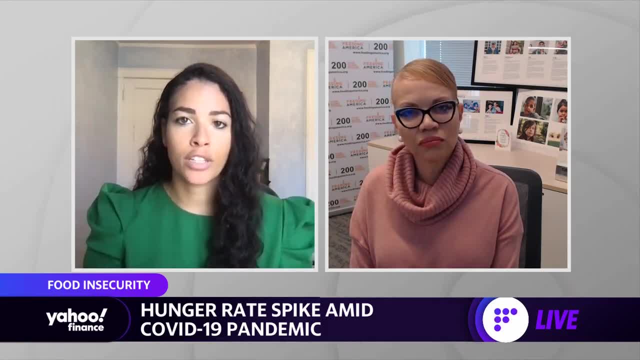 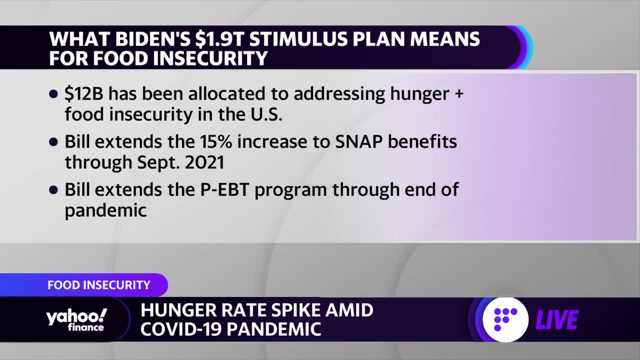 did step in in terms of stimulus, And I know that we have a graphic that has shown the impact there. I'm wondering if the stimulus is enough or not enough to tackle this problem right now and how long you think that folks are going to need to be helped. 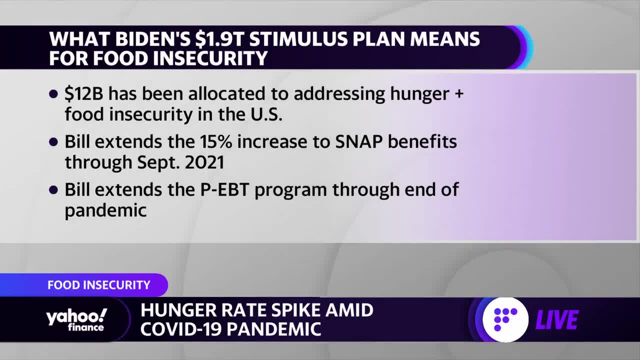 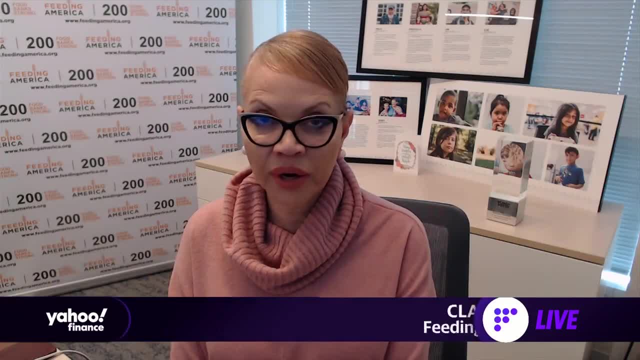 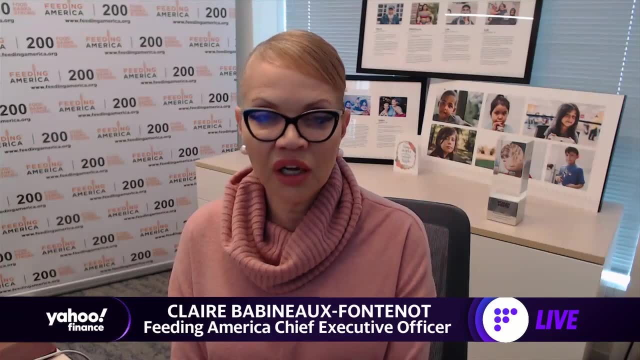 Yeah, so let me go back before the stimulus. This is one of the places where we've been able to have bipartisan support. During the previous administration there was lots of outpouring of support and outreach increases in food that was being distributed. the deregulation of 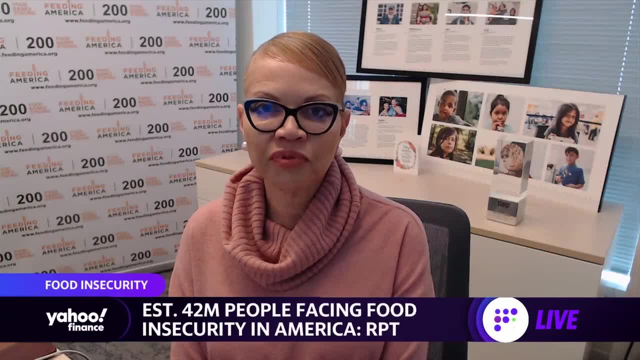 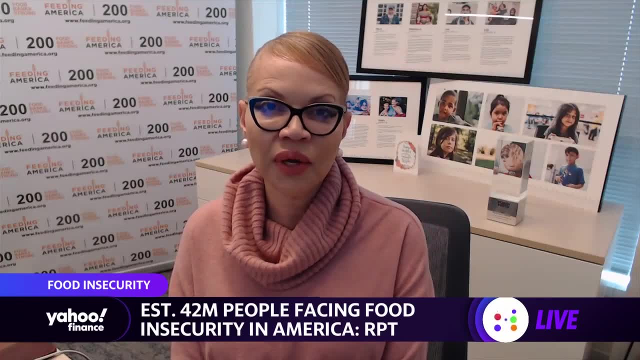 regulations that really made it challenging, especially during a pandemic, to provide food to people who needed it desperately, And we've seen that continue in this administration and we're really excited about that too. This new bill has a lot of really positive things in it. 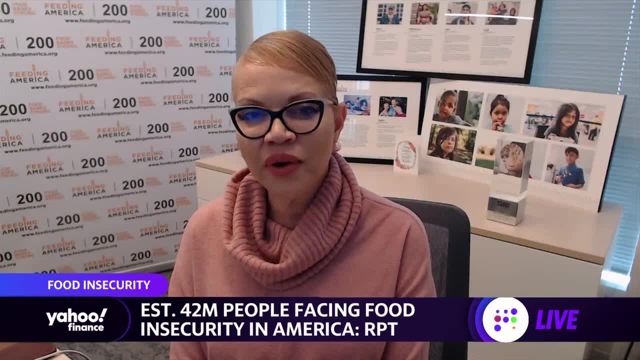 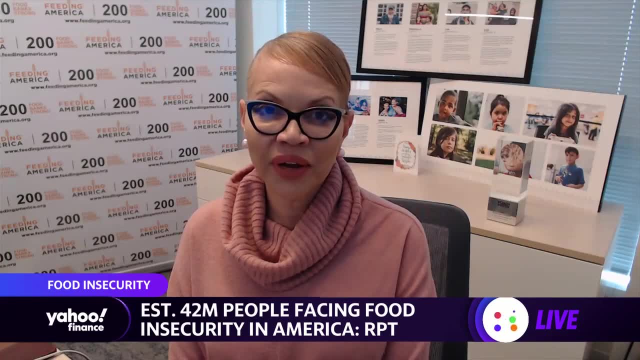 But I would tell you that most of what's being provided is temporary and that, unfortunately, if PASS is prologued, the issues are going to be won't be quite as temporary as the relief is. So we're looking at at least five, maybe 10 years of really challenging recovery for people who've 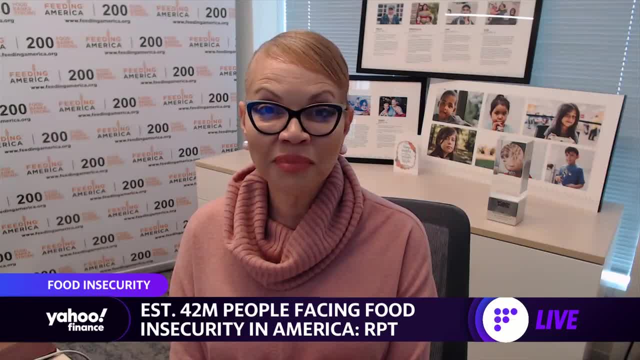 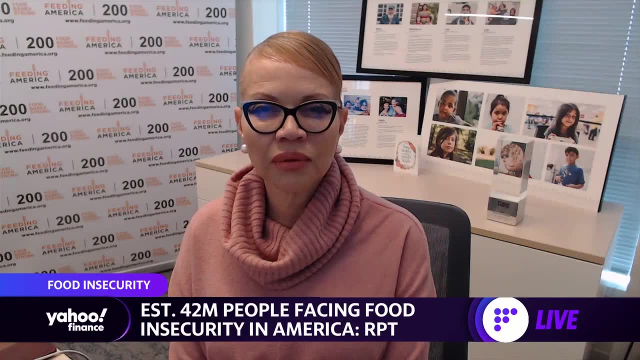 been hit hardest by this pandemic. So this is, we sometimes say it's a good down payment, but it certainly will not get us all the way to the finish line, not the 42 million people, All right. So in terms of getting to that finish line, Feeding America has launched the Food. 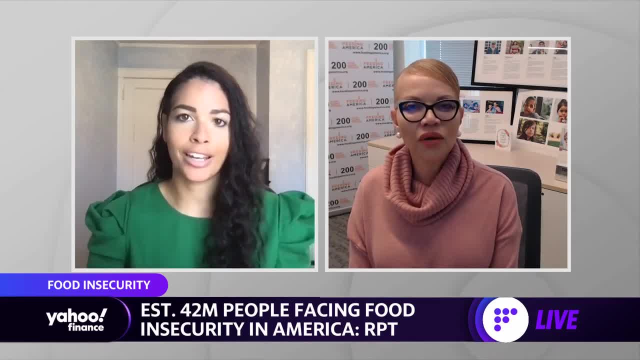 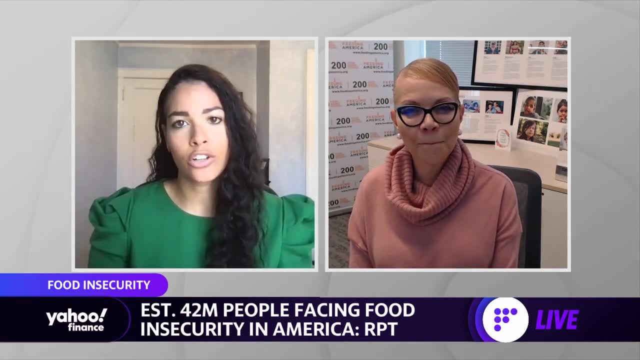 Security Equity Impact Fund. You've got some seed money- I say some, it's $20 million, which is no small feat for Mackenzie Scott- And that's going to be invested in communities of color and address the root causes of hunger. Now we've seen a lot of organizations take this route. 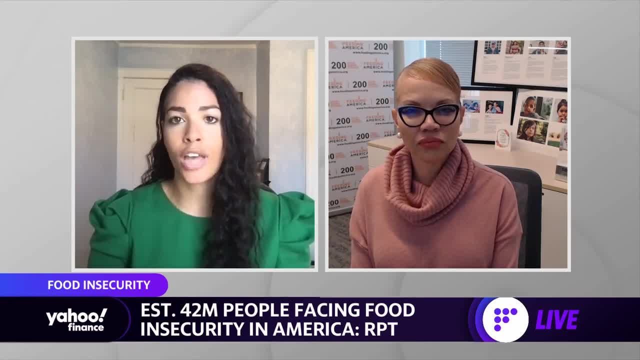 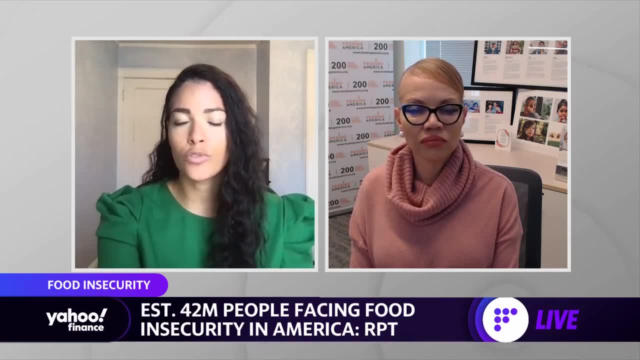 of creating funds, using investments to essentially tackle a lot of the food crisis. So I think it's a lot of worthy and worthwhile causes. How will this fund continue to drive progress in terms of reducing hunger in the United States? Yeah, well, one of the things that I hope will not be unique.